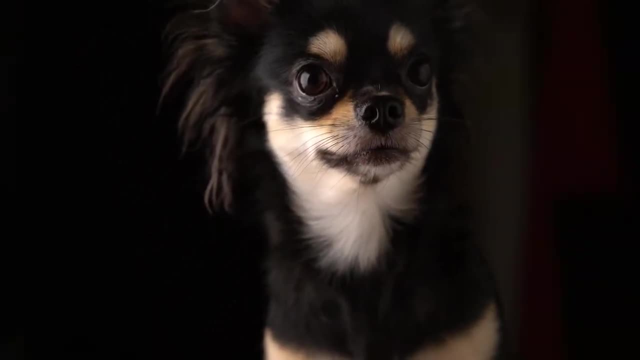 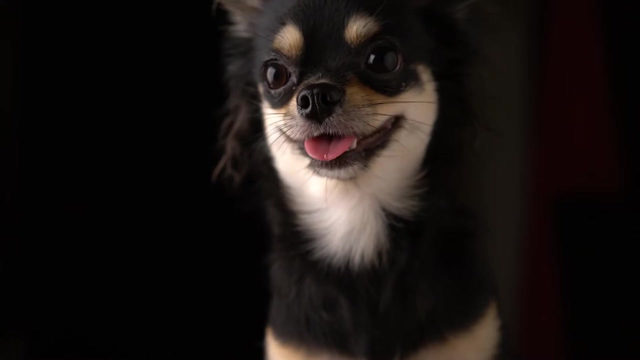 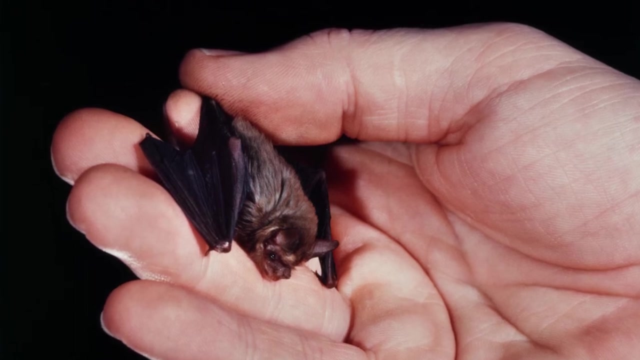 The littlest dog ever measured, was only 9.6 centimeters tall and weighed less than a kilogram. As tiny as that is, it is not even close to the smallest mammal in the world. This is the bumblebee bat, which grows to just over two centimeters in length. 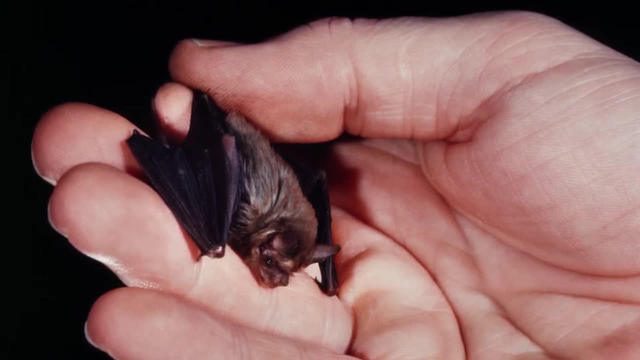 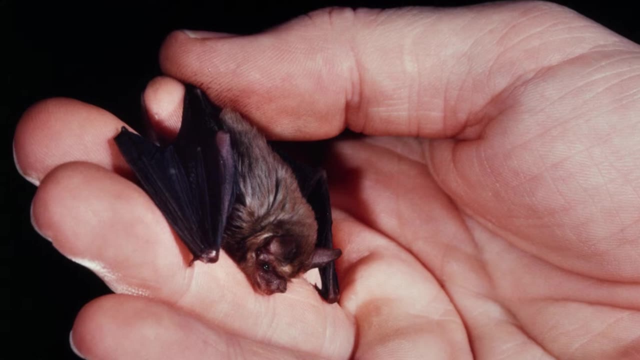 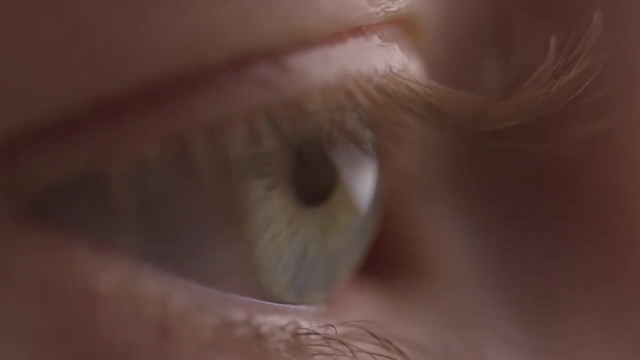 and weighs only two grams- about the weight of a single dime. Of course there are many things more minuscule than that in our world, but how can we see them? Scientists believe that the human eye, with no assistance, can see objects as small as 0.1. 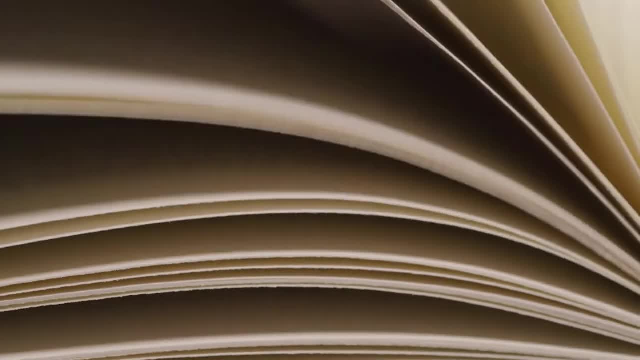 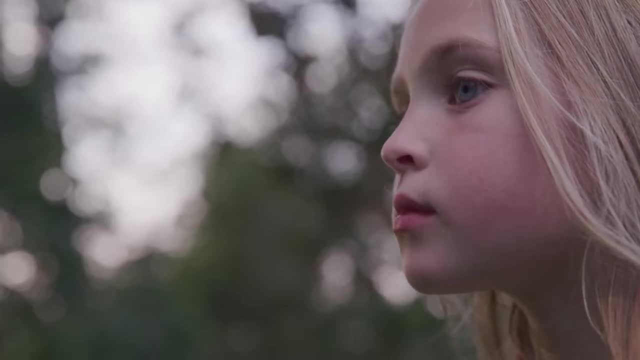 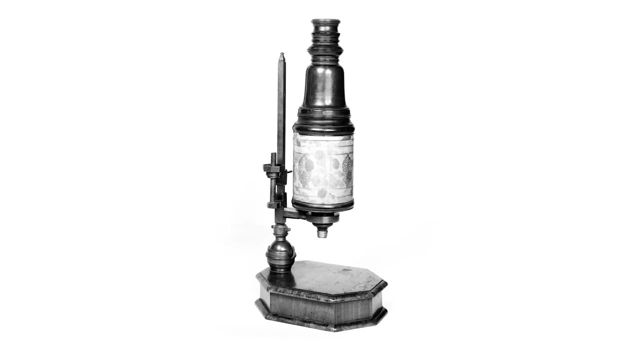 millimeters: That's about the thickness of a piece of paper, a strand of human hair or a fine grain of sand. For thousands of years, humankind was limited to observing things with only the naked eye, But that all changed with the invention of the microscope in the 17th century. 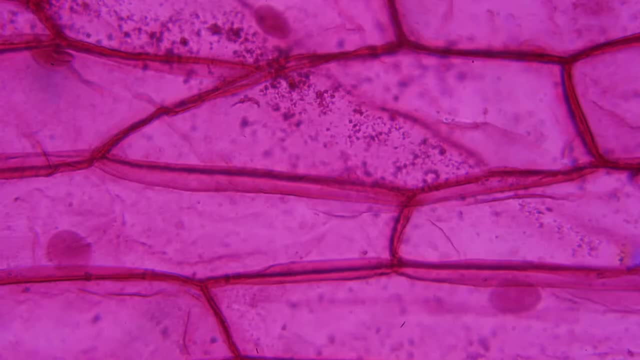 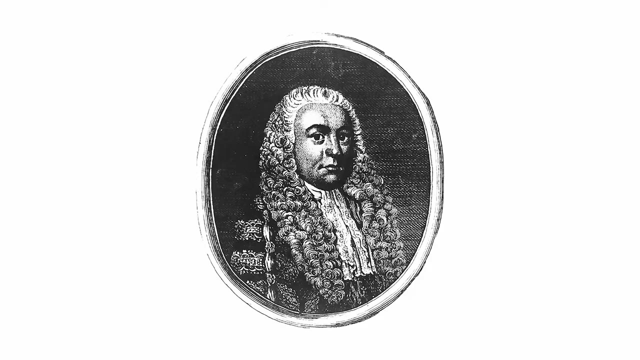 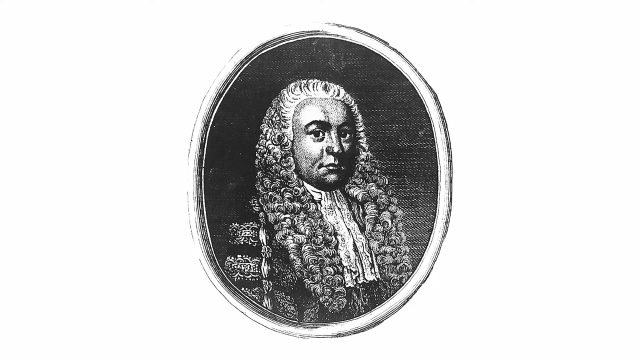 Many discoveries were made through the lens of a microscope, revealing an entire microscopic world that no one had ever seen before. In 1665, Robert Hooke, a scientist from England, was experimenting with one of the first primitive microscopes As he studied a piece of cork under magnification. 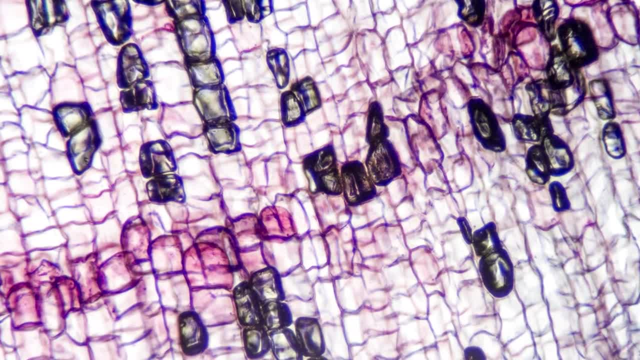 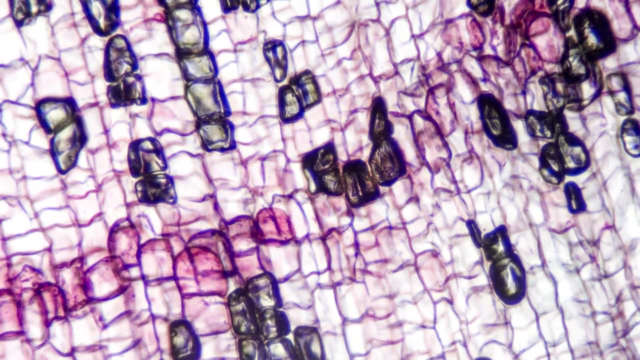 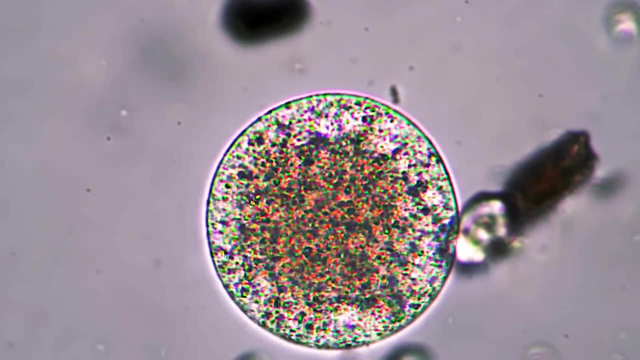 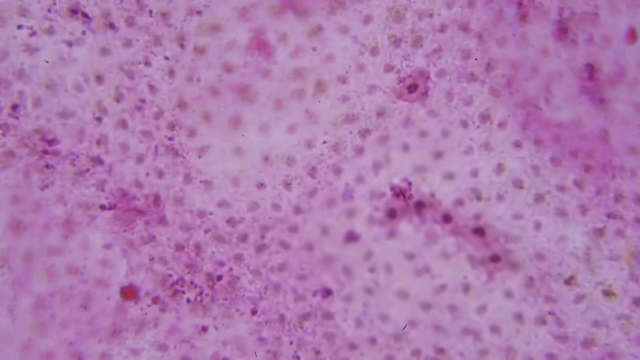 he noticed that the cork was divided into tiny microscopic sections. Hooke named these tiny divisions cells. This small discovery would change science forever. All living things are made up of these cells. They are the smallest working unit of living organisms. Because of this, cells are known as the building blocks of life. 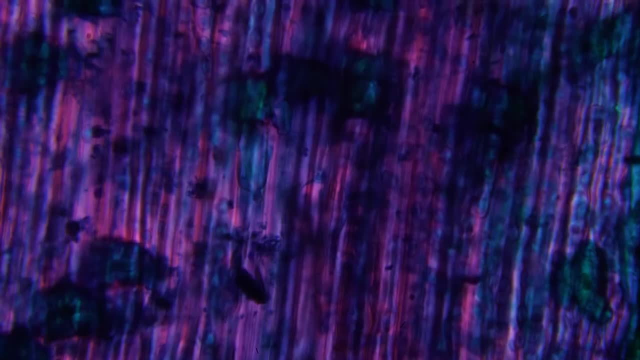 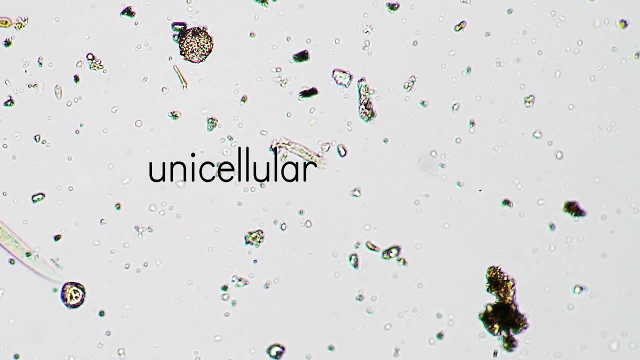 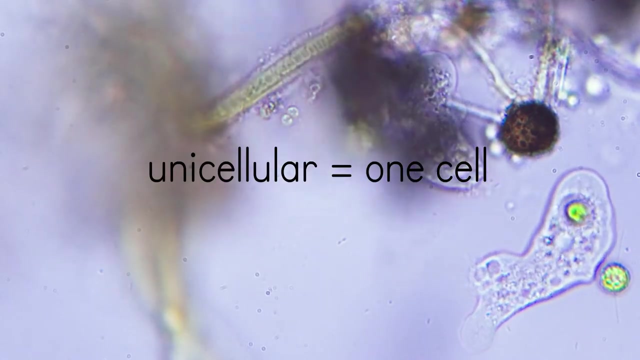 things in our world are made up of only one single cell, like this single building brick. These organisms are called unicellular, and entire kingdoms of life are made up of these one-celled creatures. Unicellular organisms are also known as microorganisms. 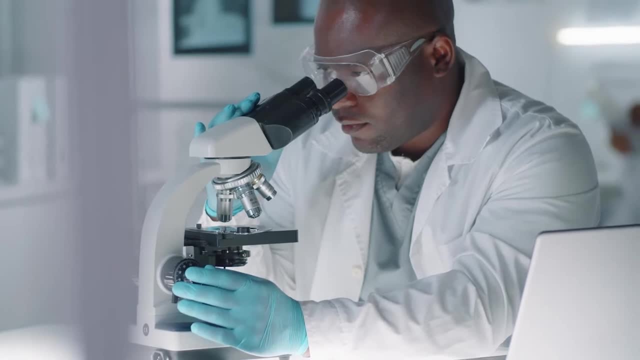 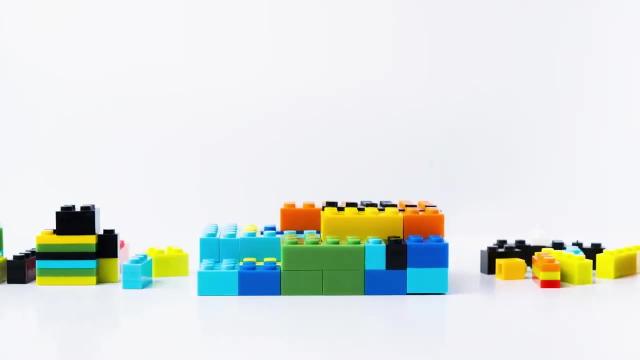 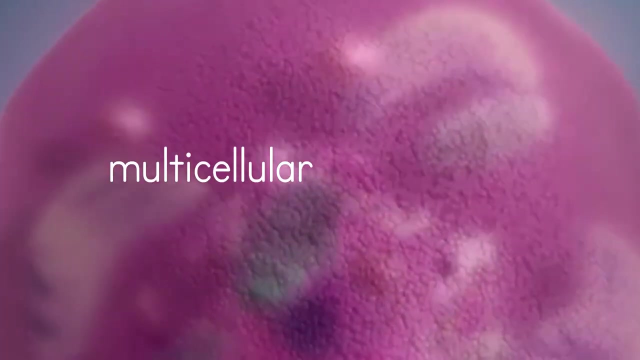 They are everywhere, but they are so small that you cannot see them without a microscope. Just as you build something bigger out of blocks, by snapping them together, cells can also be combined. The resulting multicellular organisms are much larger and more complex than unicellular. 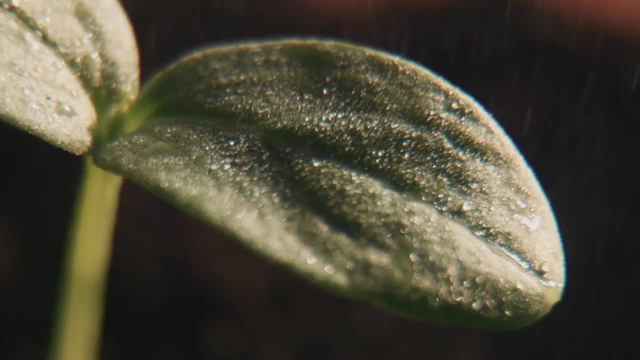 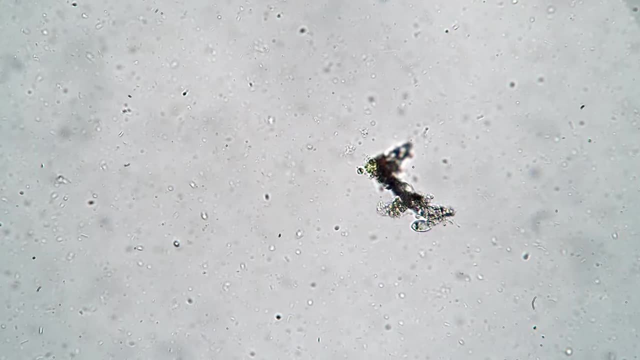 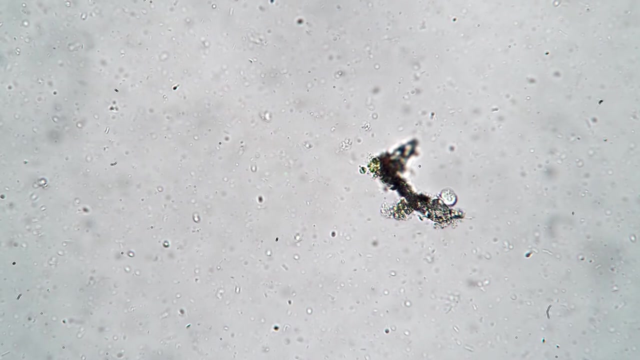 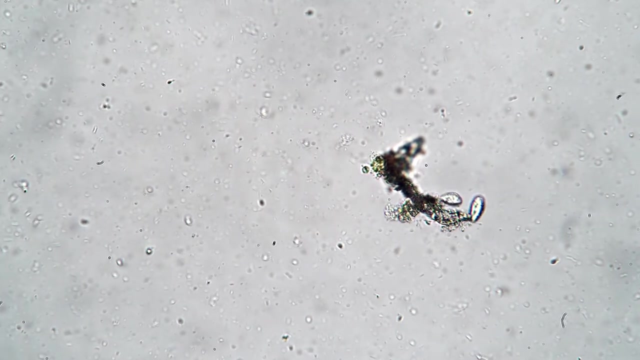 organisms. Plants and animals are examples of organisms made of many cells working together. The biggest difference between a unicellular organism and a multicellular organism is that the single-celled creature has only one vulnerable cell with no protecting cells around it. If the cell dies, the organism also dies. 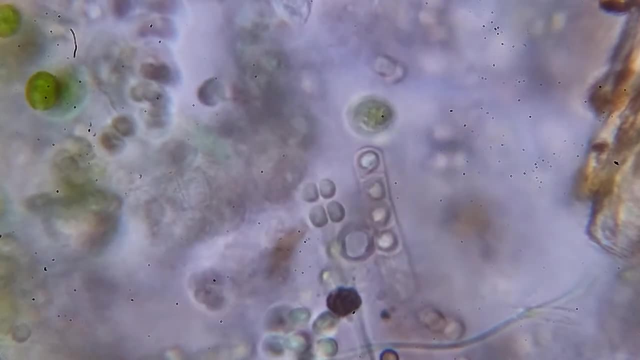 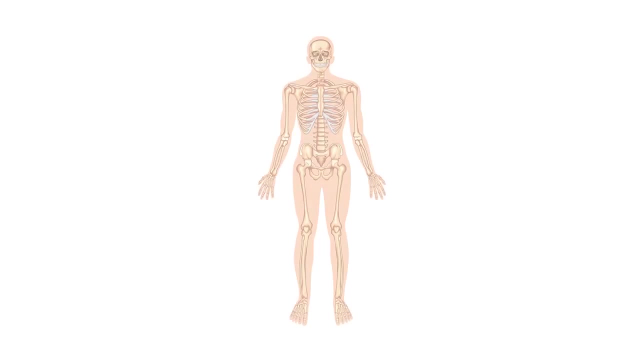 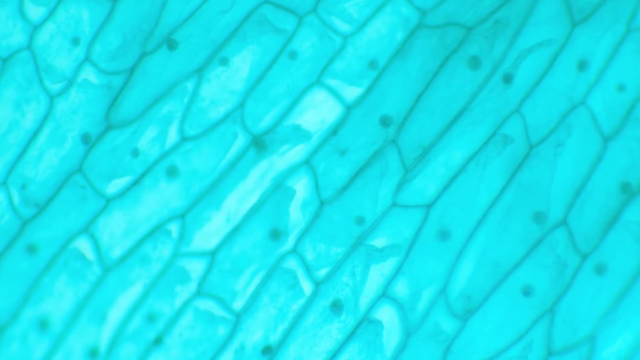 On the other hand, a multicellular organism has many specialized cells. If one cell dies, the organism can still survive. For example, the human body is made up of trillions of cells. Every second, a million of them die and are replaced by new cells. 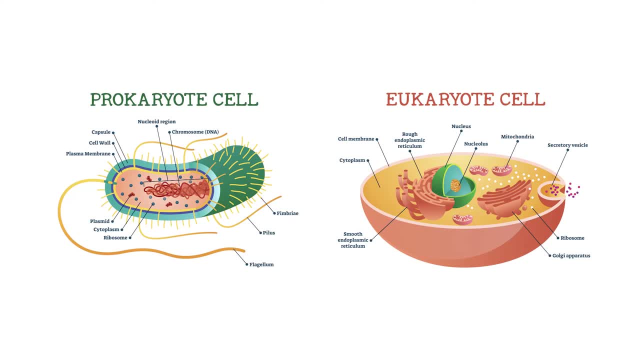 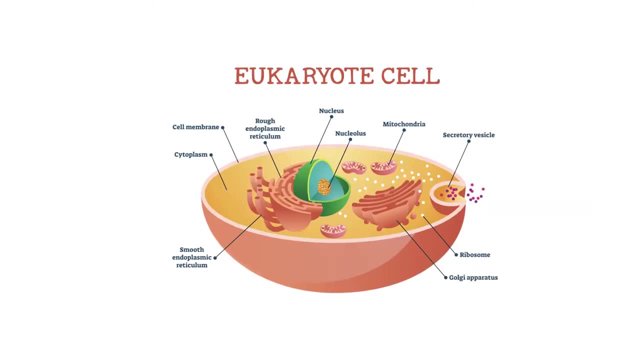 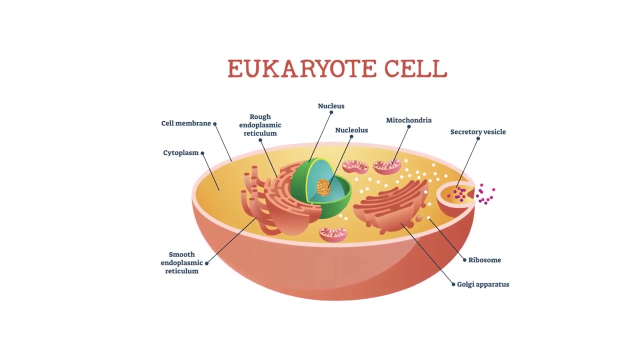 There are two defining types of cells on Earth: prokaryote and eukaryote. The main difference between these two types of cells is that eukaryotic cells have specialized organelles, including a membrane-bound nucleus. An organelle is a membranous structure inside the cell. 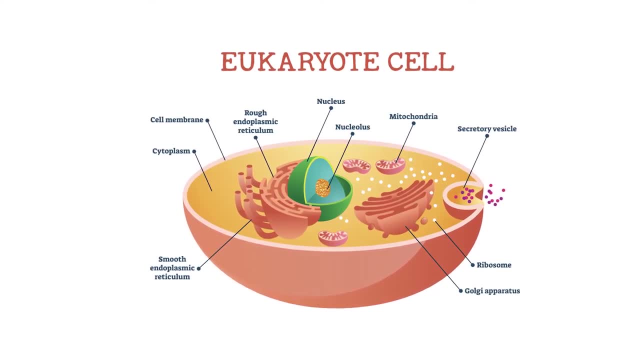 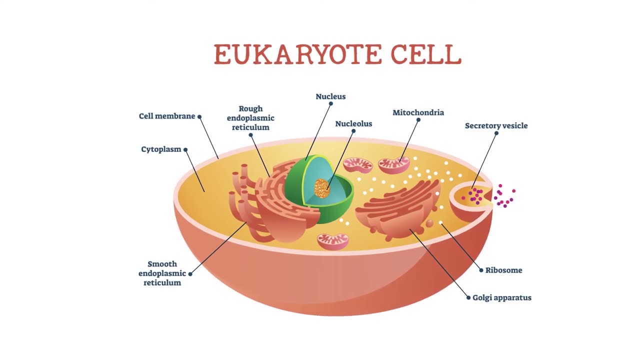 The organelle is a membrane-bound nucleus. An organelle is a membranous structure inside the cell. The organelle is a membrane-bound nucleus. This is the part of the cell that performs a specific job, And the most important organelle in a eukaryotic cell is the nucleus. 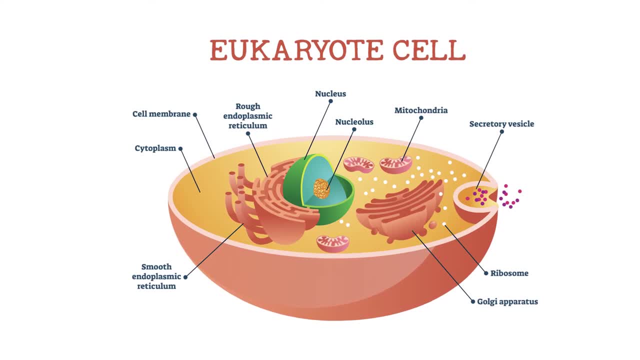 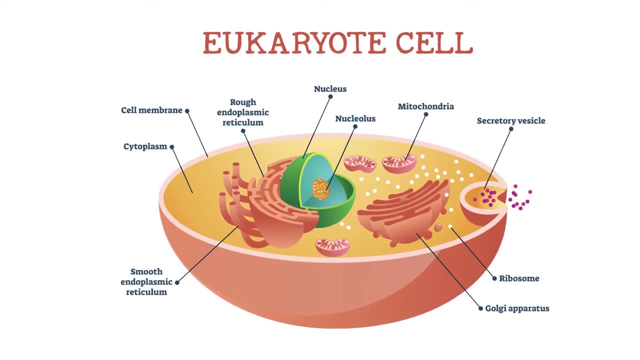 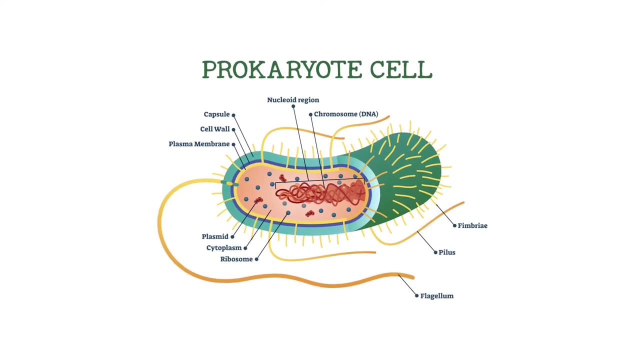 The nucleus contains the genetic material for the cell and is the control center, similar to a brain, directing the cell's activities and functions. The genetic material of the prokaryote floats freely within the cell's cytoplasm, along with organelles less complex than those found in the early human species. 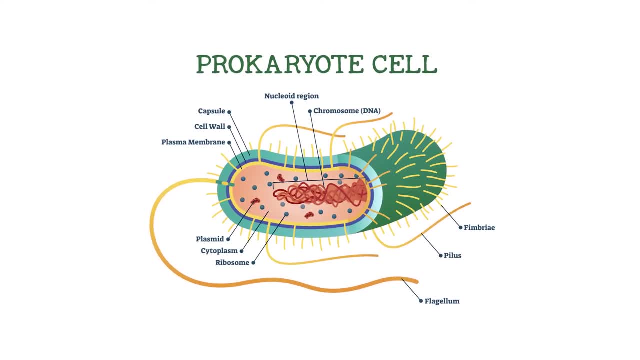 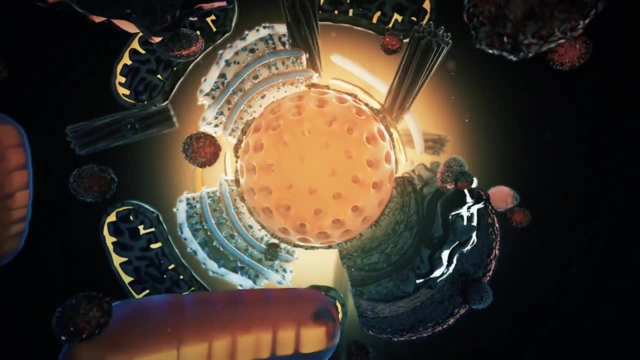 It is the human body that has the most important organelle under its control- and the cell's- than those found within a eukaryote. the cell is the most basic part of your body and is part of an amazing organizational system. a single cell joins together with: